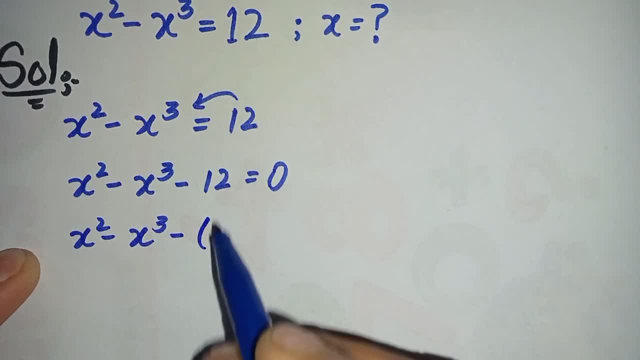 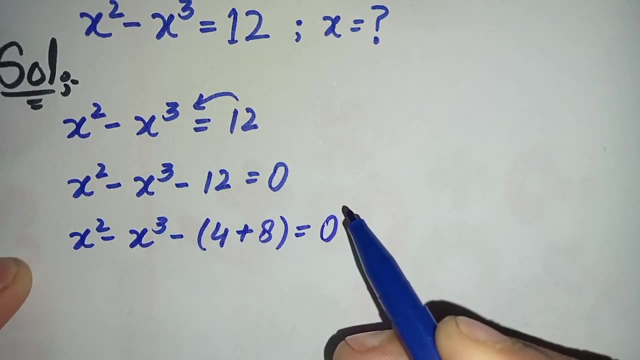 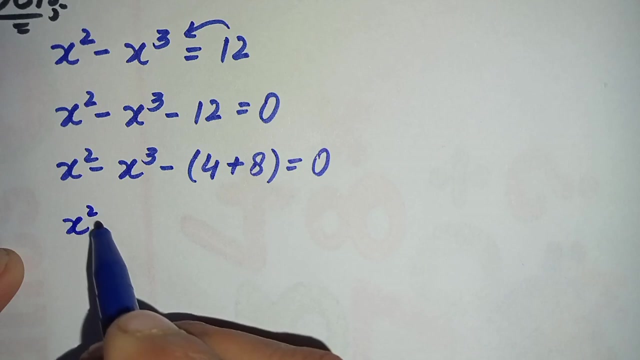 x cube minus. we can write this: 12 as 4 plus 8 is equal to 0.. In the next tip we will multiply this negative side, inside the parentheses: x square minus x cube will become minus 4 minus 8 is equal to 0.. 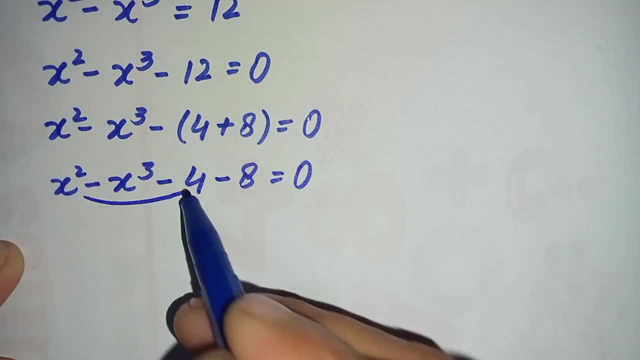 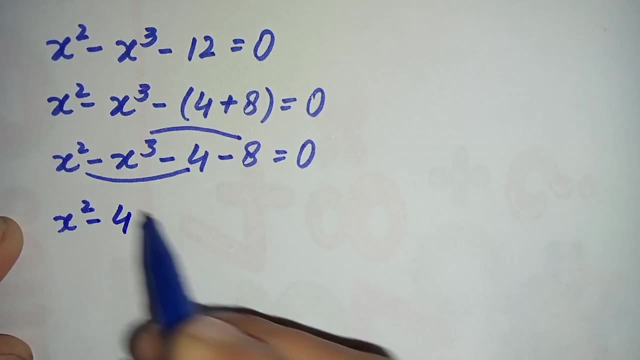 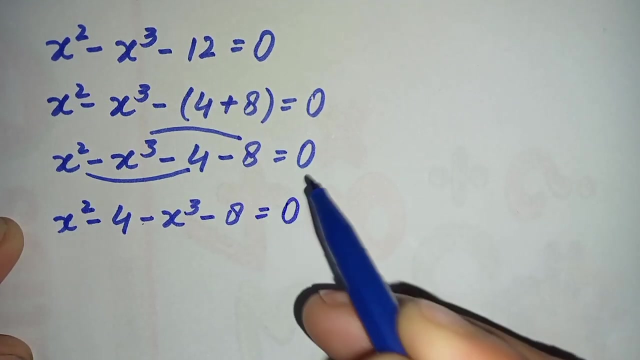 In the next tip we will combine this x square with 4 and this x cube with 8.. So it will become x square minus 4 minus x cube minus 8 is equal to 0.. Now here we will change this 4 and this 8 to its exponential. 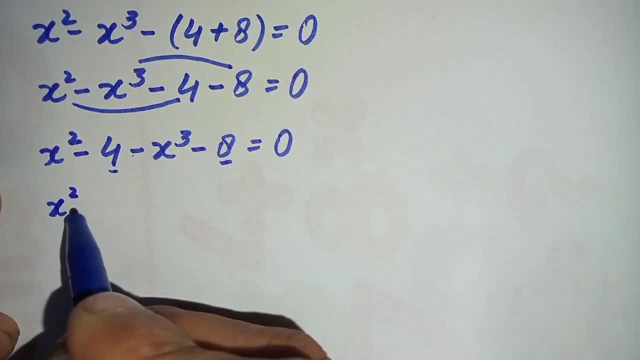 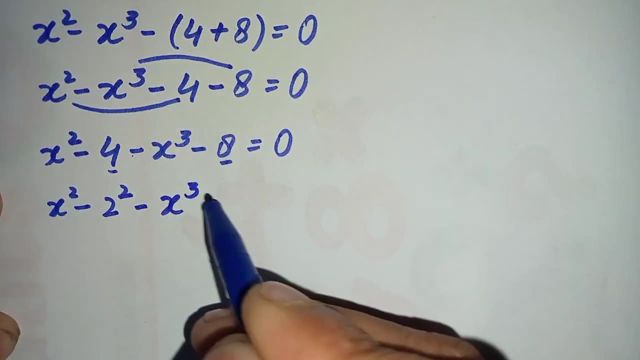 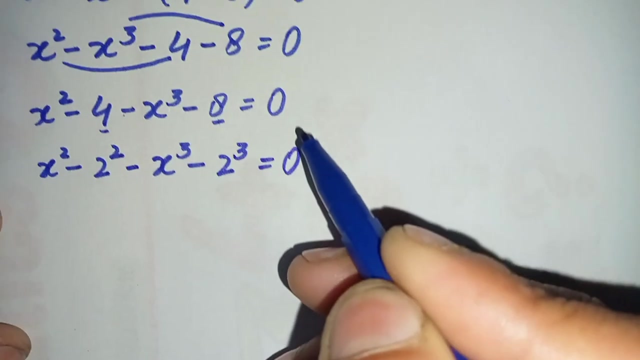 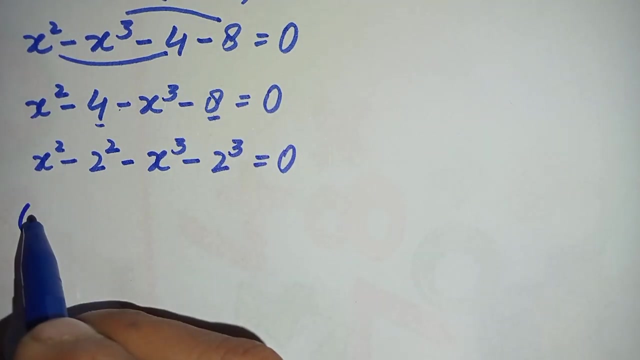 form. So we can write the exponential form as minus, or can be written as 2 square minus x cube minus 8 can be written as 2 cube is equal to 0.. Now here we will combine these two terms and these two terms So we can write them as x square minus 2 square, and from this 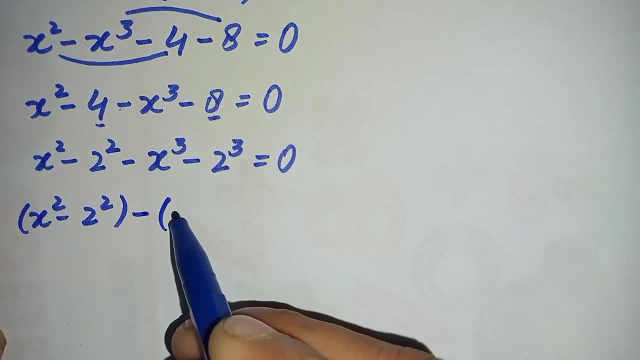 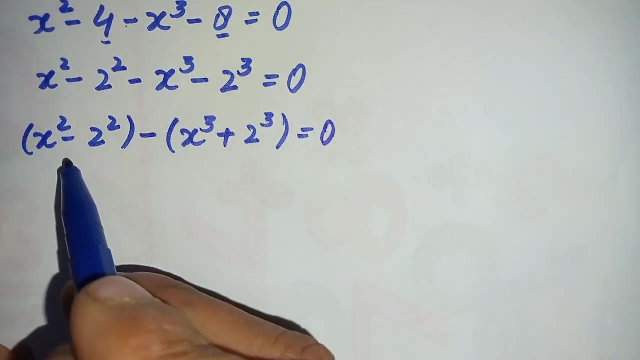 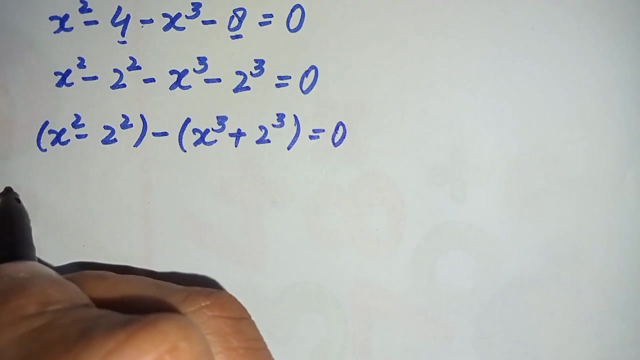 two terms. we will take negative sign comma, So it will become x cube plus 2 cube is equal to 0. Now here, in these two terms, we will use two different algebraic math formulas. So here we will use these two algebraic math formulas. Formula number one which we will use here, that is: 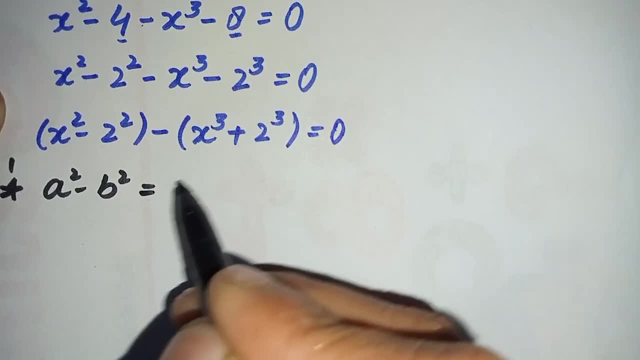 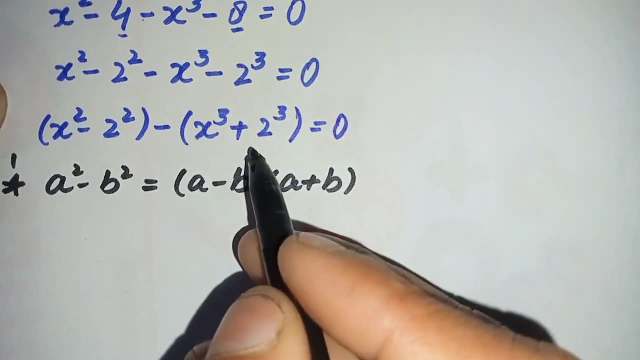 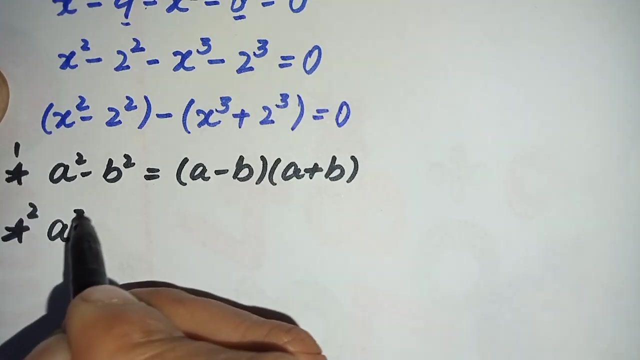 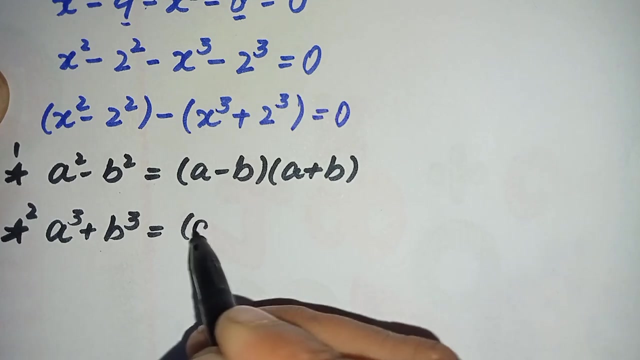 a square minus b square is equal to a minus b times a plus b, And here we will use a cubic algebraic identity. So we will use this identity here. a cube plus b cube can also be written as a plus b times a square. 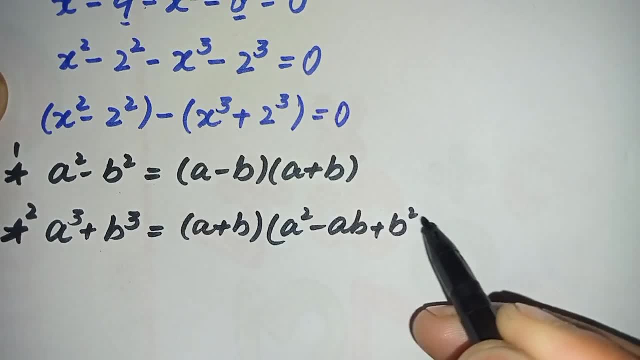 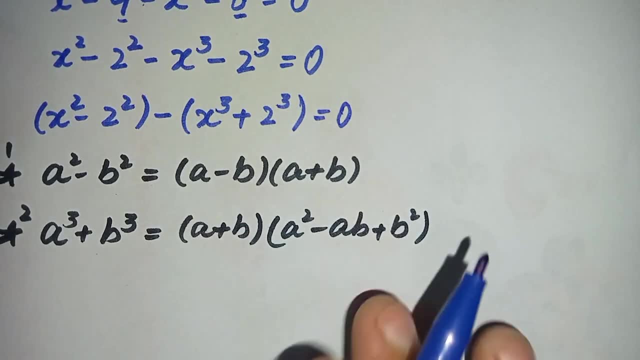 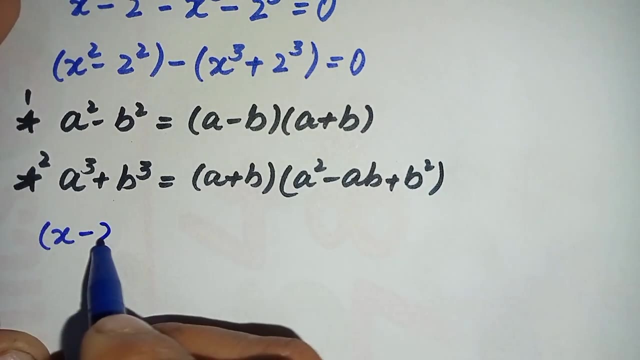 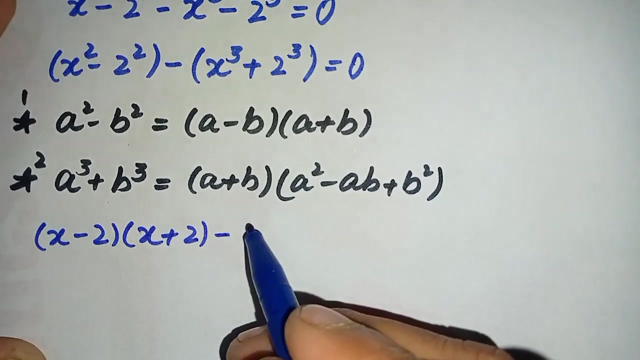 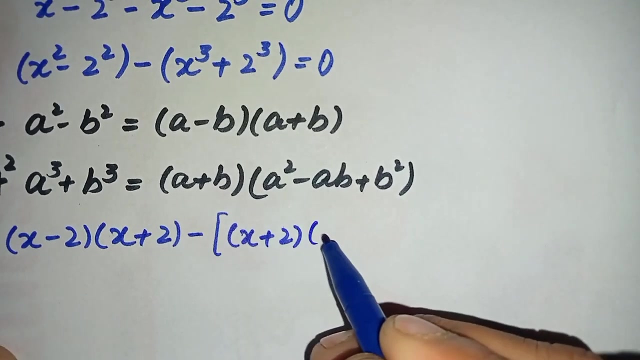 minus a b plus b square. so by using these two different algebraic identities in this one equation, this equation will become here: this term will become x minus 2 times x plus 2 minus, and it will become x plus 2 times x square minus 2x. 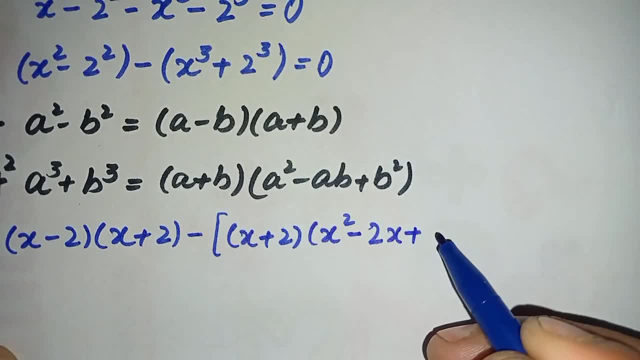 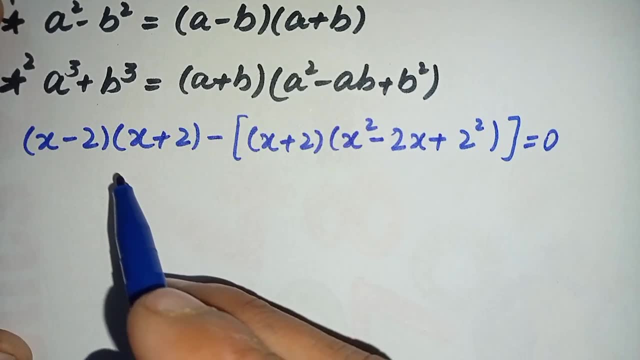 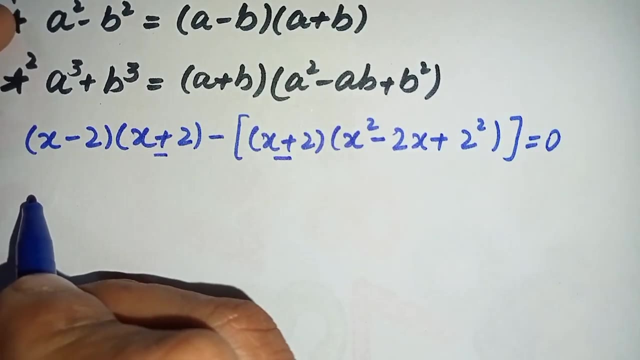 plus b square, that is 2 square number dear's. look into this equation. number dear's. look into this equation. number dear's, look into this equation. from here: we will take x plus 2 common. from here we will take x plus 2 common. from here we will take x plus 2 common from both the terms. so it will become: 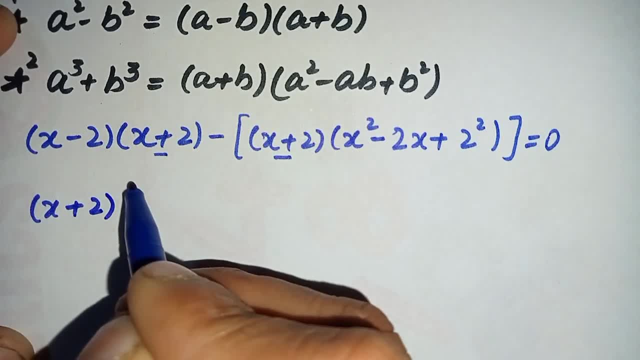 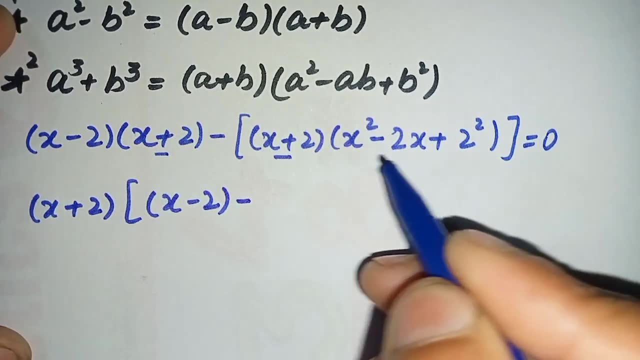 from both the terms. so it will become from both the terms. so it will become taking x plus 2 common, so here x minus 2. taking x plus 2 common. so here x minus 2. taking x plus 2 common. so here x minus 2 is left minus and here only this one. 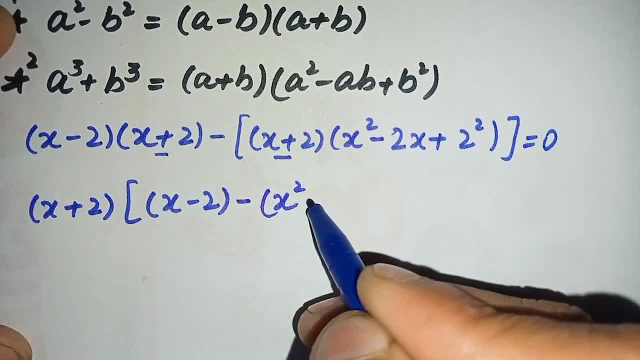 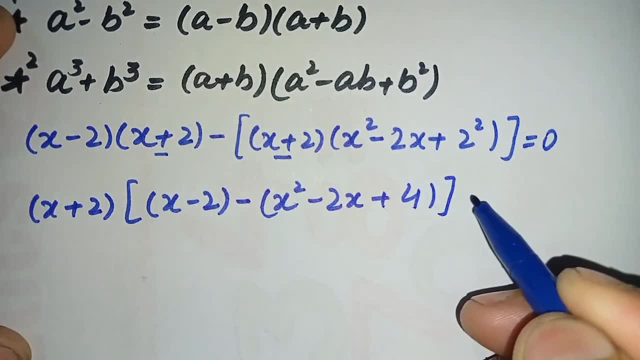 is left minus, and here only this one is left minus and here only this one expression is left: x square minus 2x. expression is left. x square minus 2x. expression is left: x square minus 2x plus 2. square is equal to. 4 is equal to. 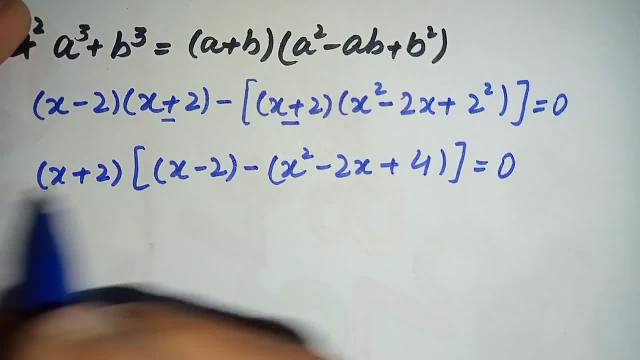 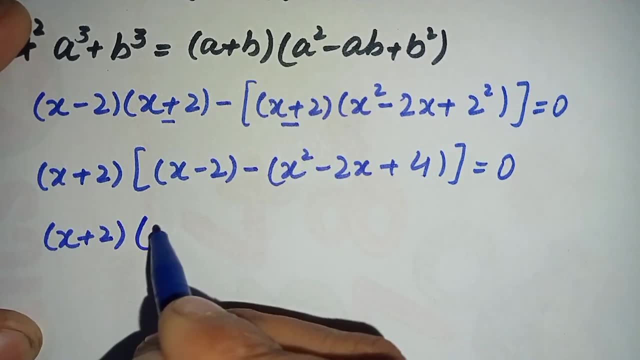 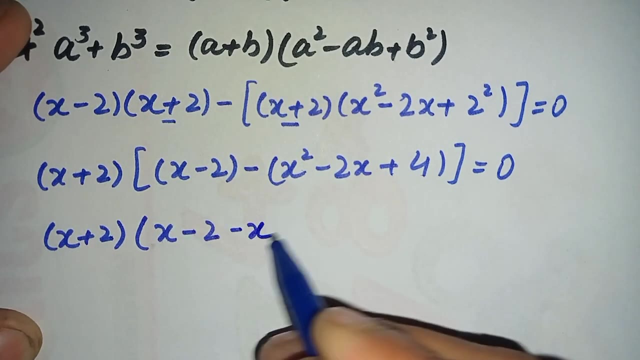 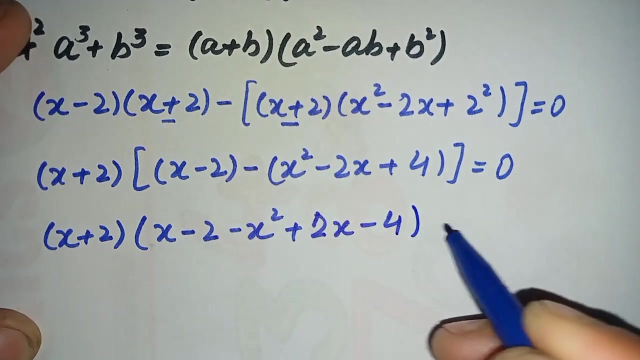 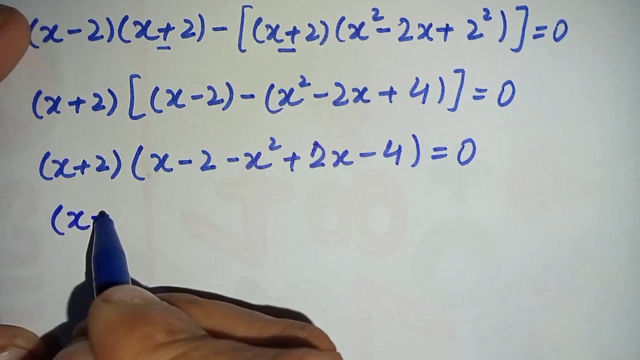 plus 2 square is equal to 4, is equal to zero. so let's further simplify this equation. this expression: x plus 2 times it will become x minus 2. we will multiply this negative sign inside the parenthesis. that will become minus x. square plus 2x minus 4 is equal to 0. let's further simplify this expression: x plus 2 times minus x, square x. 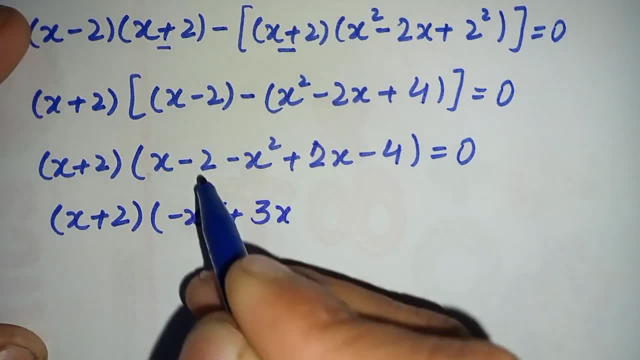 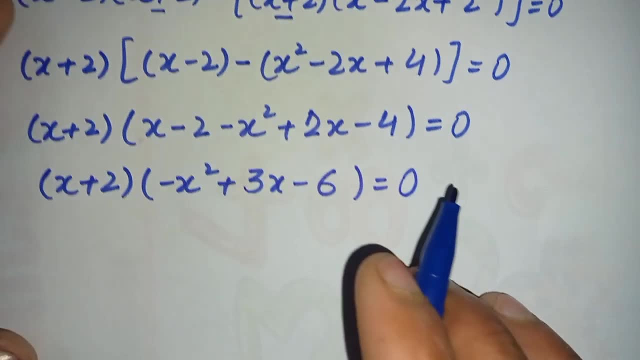 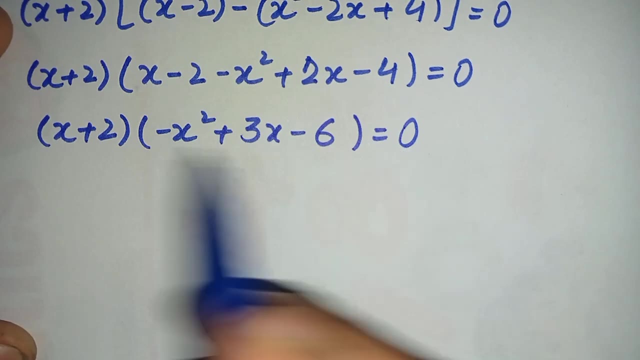 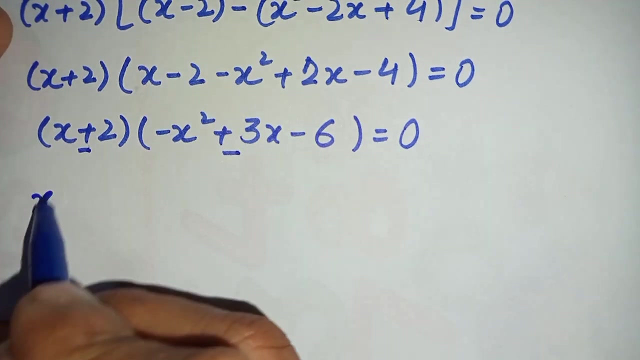 plus 2, x is 3x, minus 2. minus 4 is minus 6 is equal to 0. now, my dears, look it to this equation. here the product of these two expression is zero. so here either this expression will be zero or this one will be zero. so we can write this equation as: x plus. 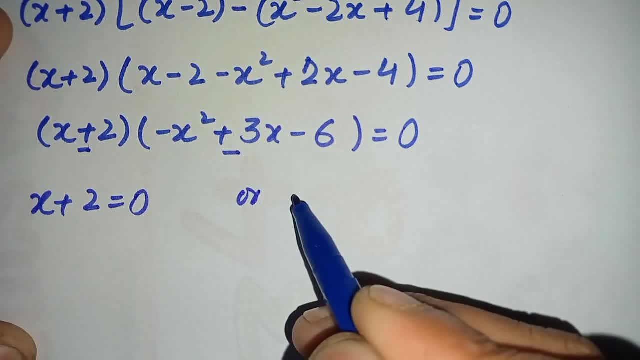 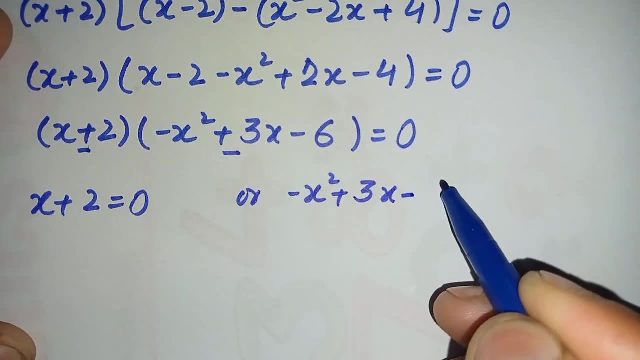 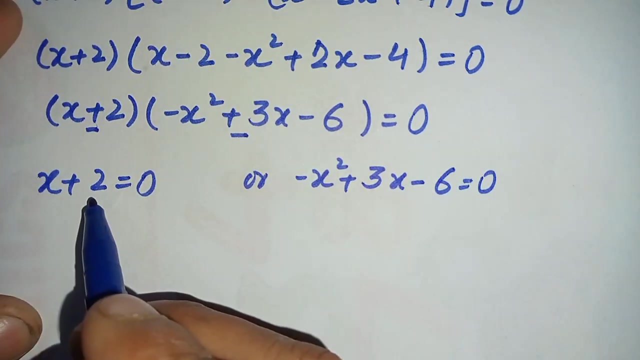 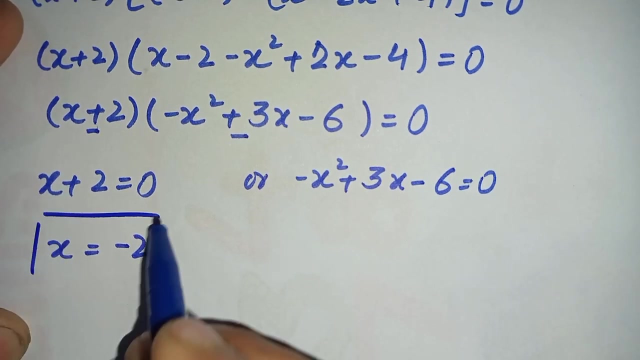 2 will be 0 or minus x. square plus 3x minus 6 will be 0. so first we will solve this one equation here. we will shift this positive 2 to the right hand side, so it will become negative 2, and this is our first real solution of the given expression equation. 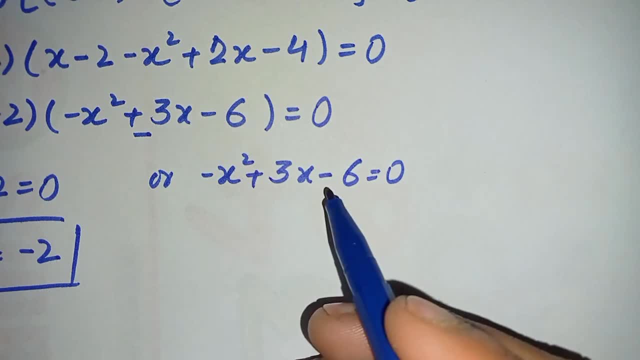 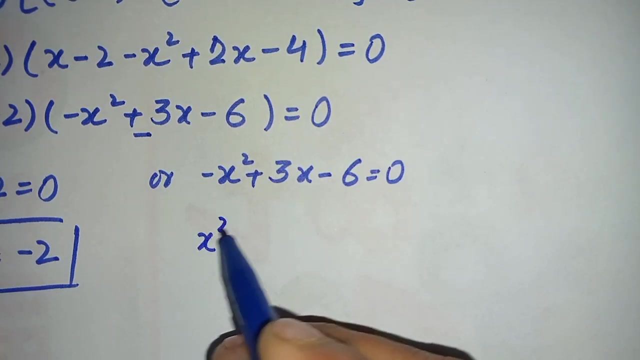 now we will solve this second equation. now to solve this equation first, we will make the coefficient of x square positive. now, to make it positive, we will multiply both sides by minus one. so by multiplying both side by minus one, we will get x square, it will become minus 3x and it will become plus. 6 is equal to 0. now we 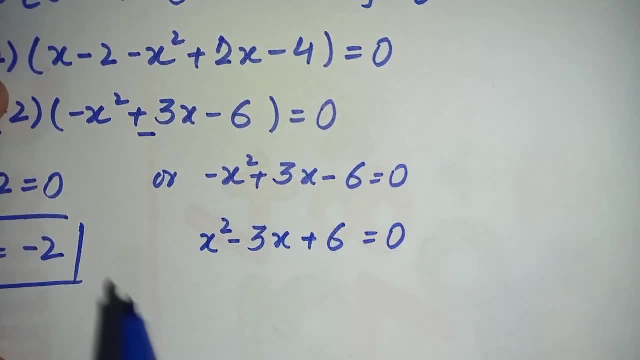 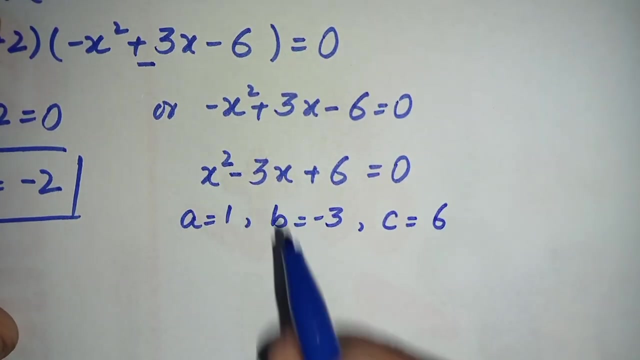 will solve this quadratic equation by quadratic formula. so here the values of a is 1, the value of b is minus 3 and the value of c is 6. so the quadratic formula for variable X is x is equal to minus b plus minus square root of b, square minus. 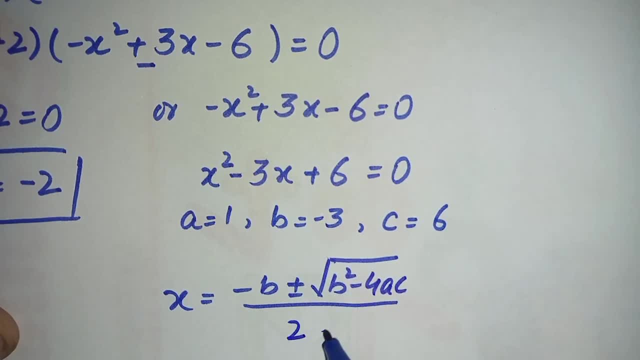 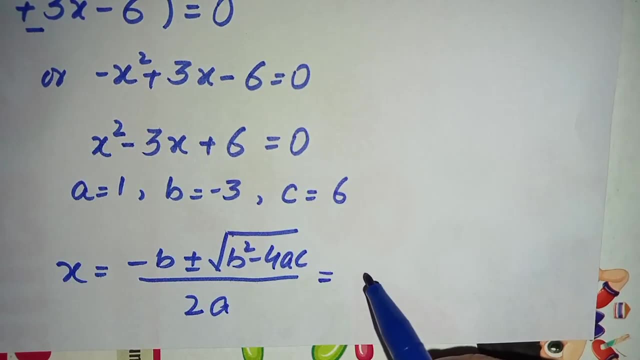 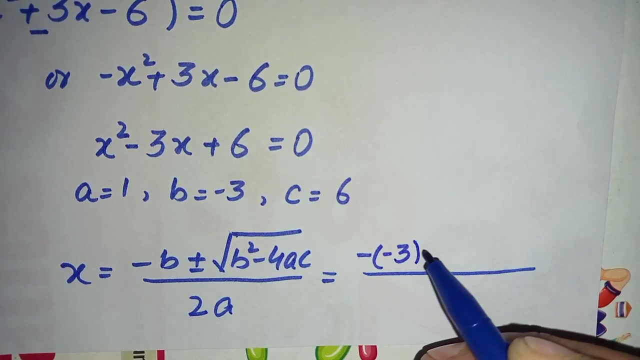 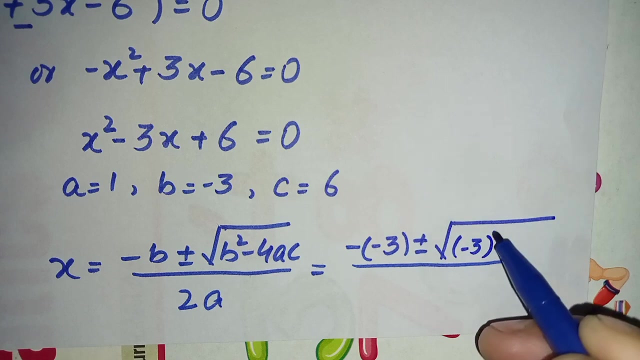 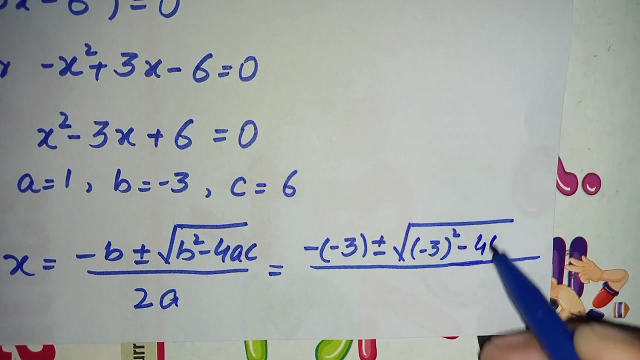 per AC divided by 2k. so here we will substitute the values of ABC from here, so it will become minus B. the value of minus B is B is minus 3 plus minus square root of b square, that is minus 3 square minus 4ac, minus 4ac. 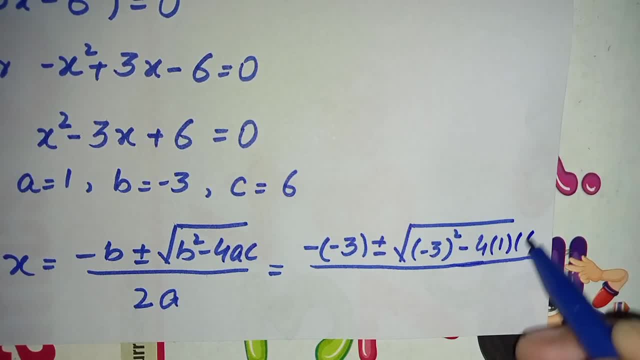 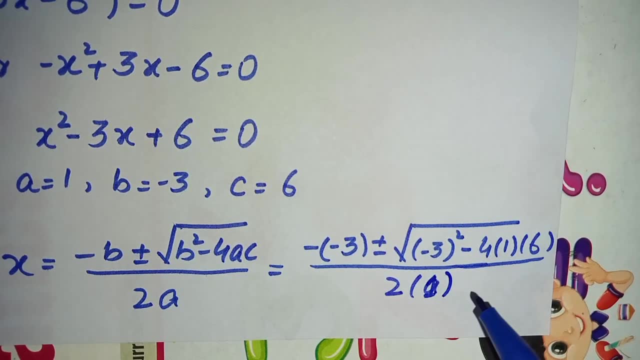 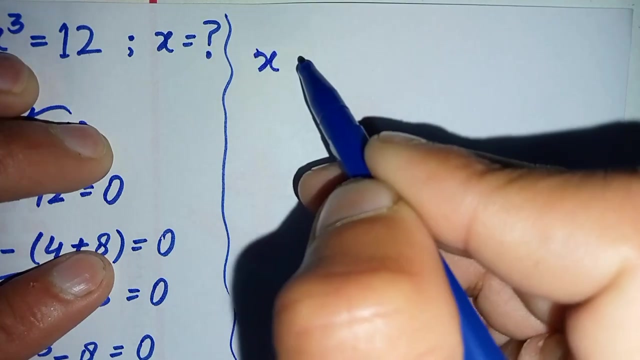 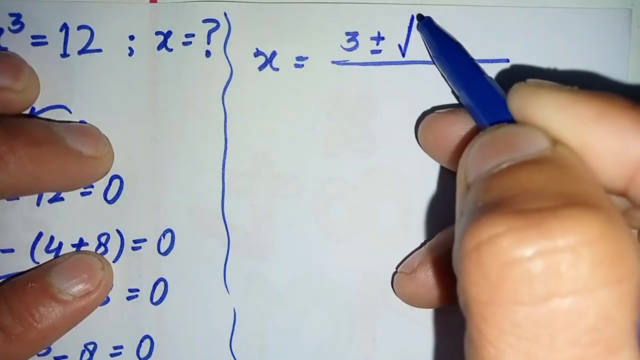 the value of a is 1 and the value of c is 6. divided by 2a, the value of a is 1. now we will do further steps here, so our last equation will become: x is equal to minus minus plus 3 plus minus square root of minus 3 square is equal to 9. 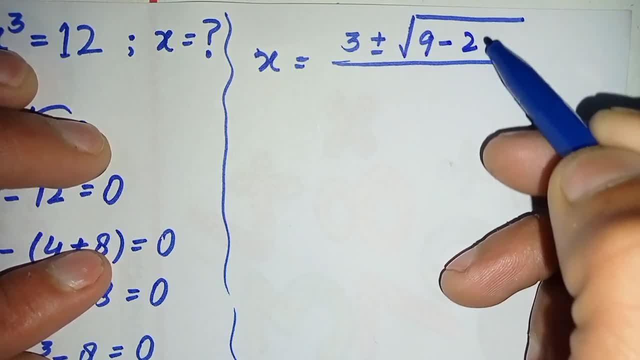 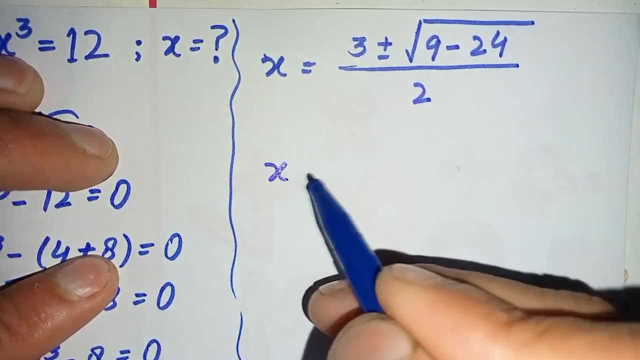 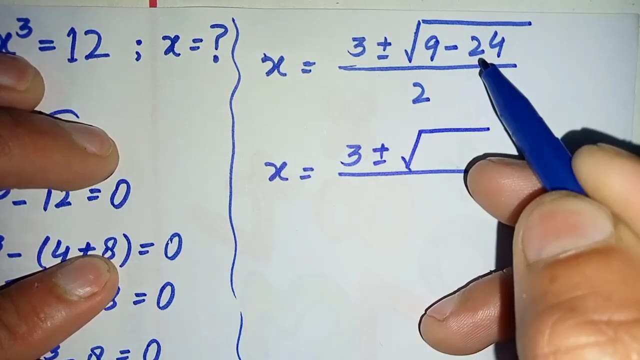 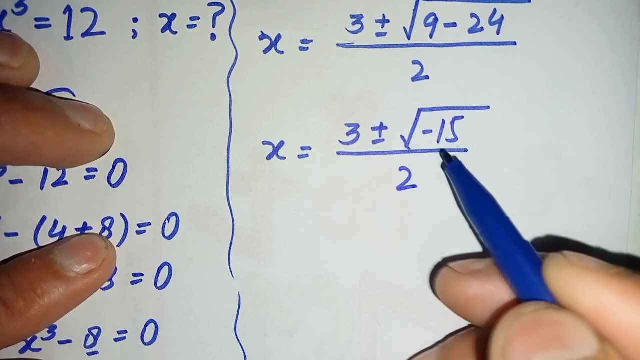 minus 4 times 1 is 4. 4 times 6 is 24. divided by 2 times 1 is 2, so further it will become: x is equal to 3 plus minus. square root of 9 minus 24 is minus 15 divided by 2. now we can write. 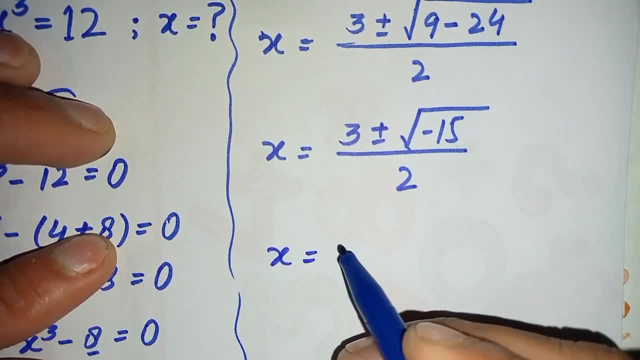 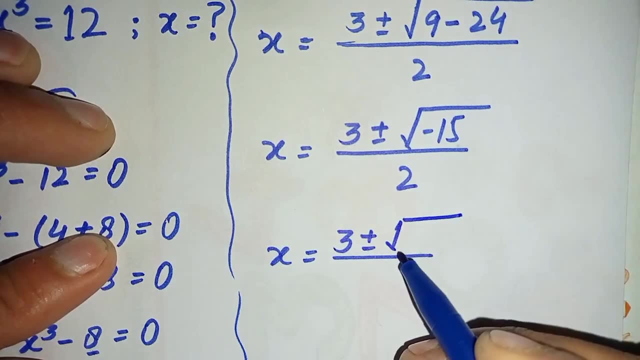 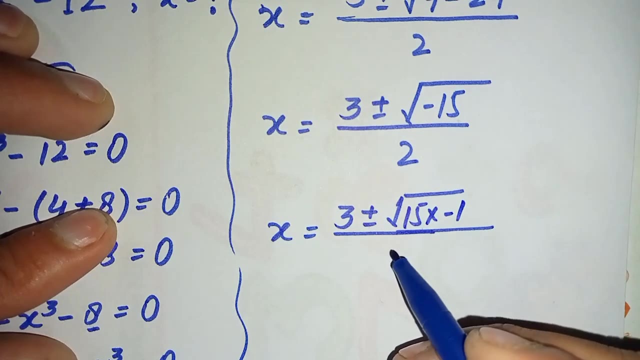 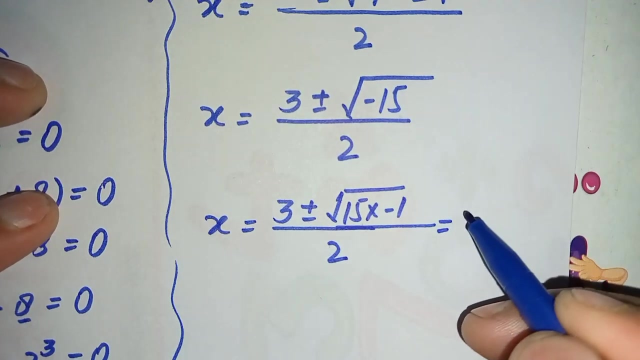 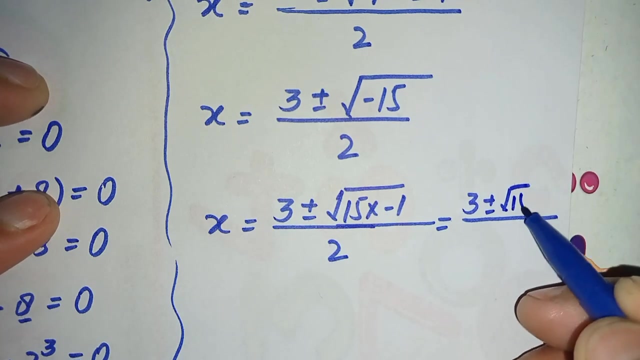 this further: as x is equal to 3 plus minus square root of, we can write this: minus 15 s, 15 times minus 1 divided by 2. in the next we will split this square root over 15 and minus 1, so it will become 3 plus minus square root of 15 times square root of minus 1. 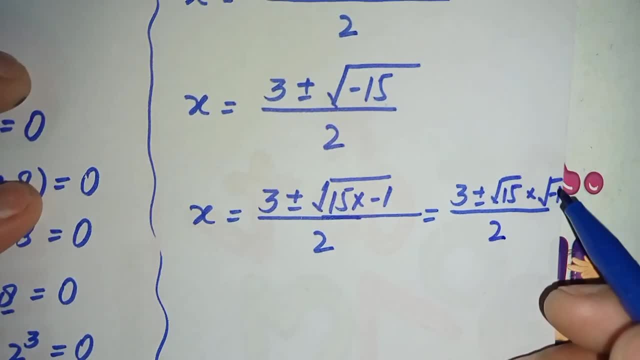 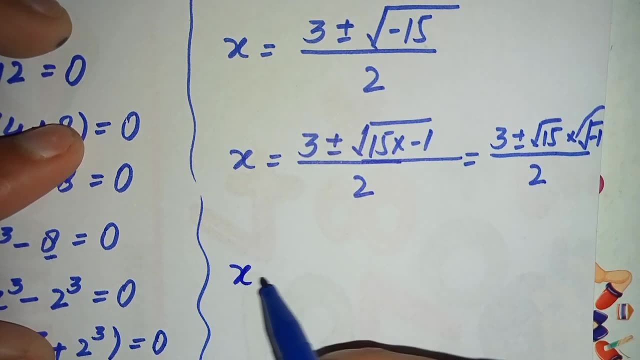 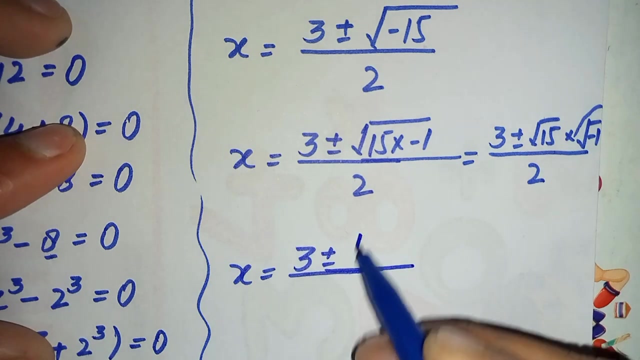 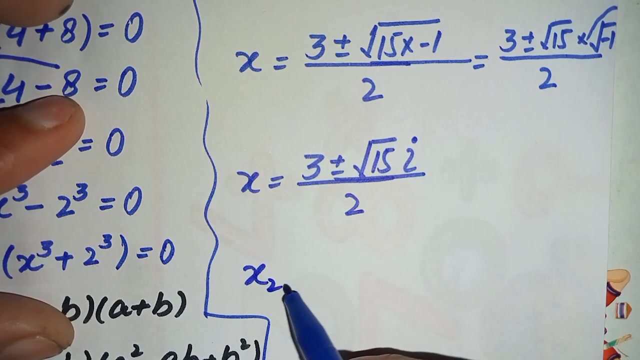 divided by 2. so here square root of minus 1 is the complex identity iota, so it will become equal to 3 plus minus square root of 15 and square root of minus minus iota i divided by 2. so these are two solutions, two complex solutions, so x2 will become 3 plus square. 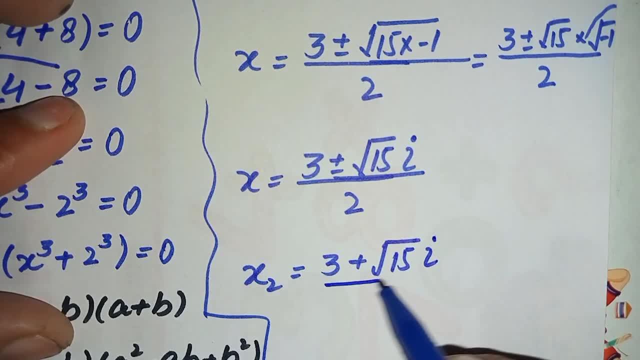 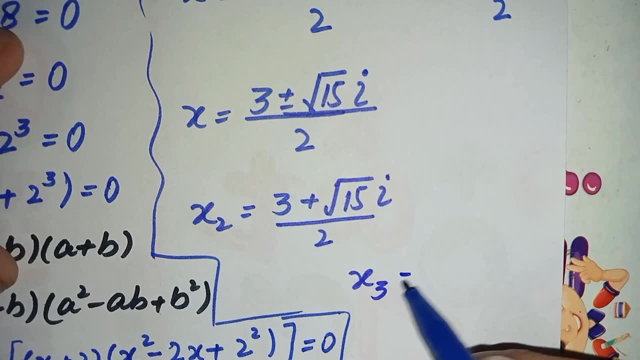 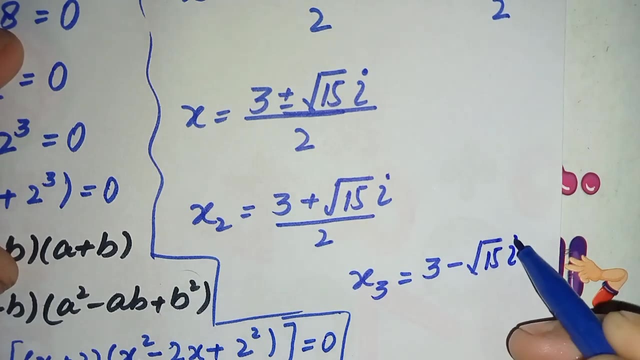 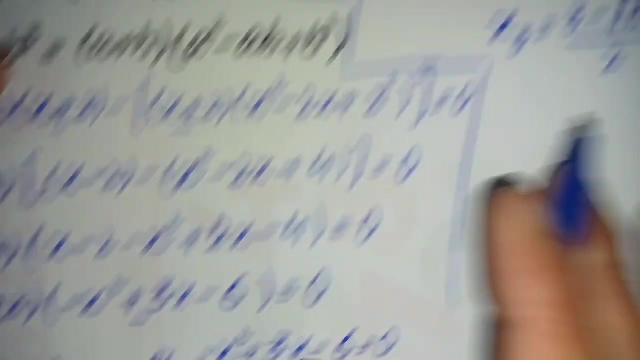 root of 15 iota divided by 2, and x3 will become 3 minus square root of 15 iota divided by 2. so finally, x1 equal to minus 2 is the real and x2 equal to 3 plus square root of 15 iota. 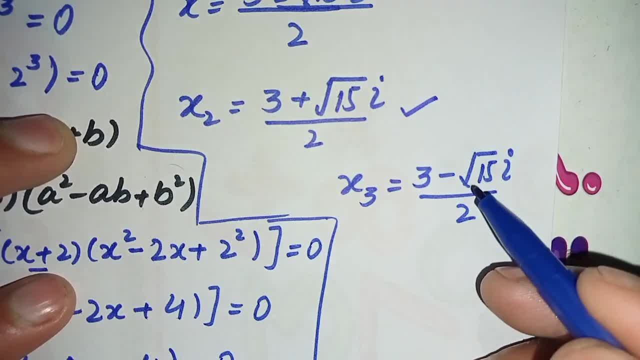 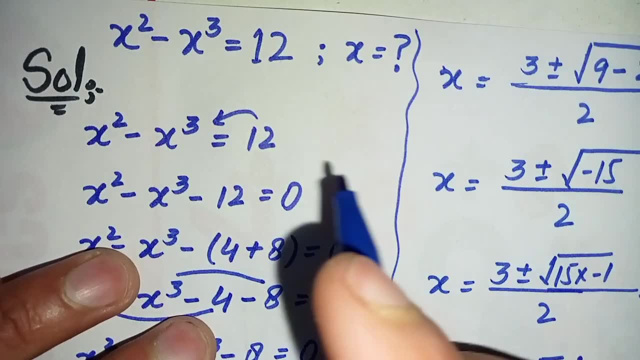 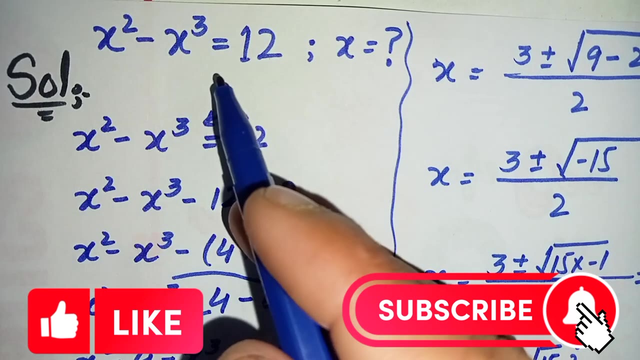 divided by 2.. and x3 is equal to 3 minus square root of 15 iota divided by 2 are the complex solutions and roots of this nice exponential equation. and last, don't forget to subscribe our youtube channel for such a more interesting math videos. thank you so much for watching. take care, see in the next video. bye, bye.